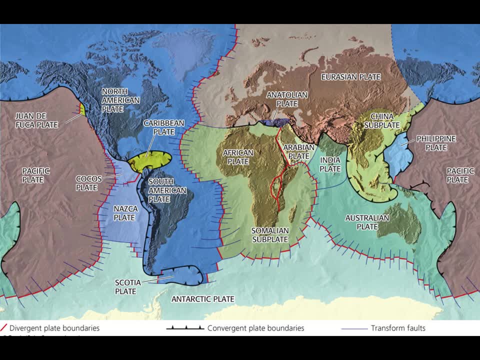 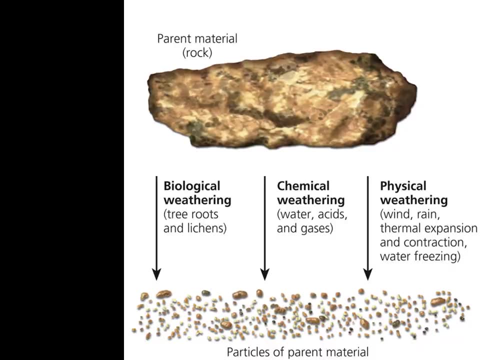 of plate boundaries like this, we can determine the location of volcanoes, island arcs, earthquakes, hot spots and faults. On the other hand, external geological forces are things that are driven by factors outside of the earth. A major example of this is weathering, where rock materials can be broken down into small 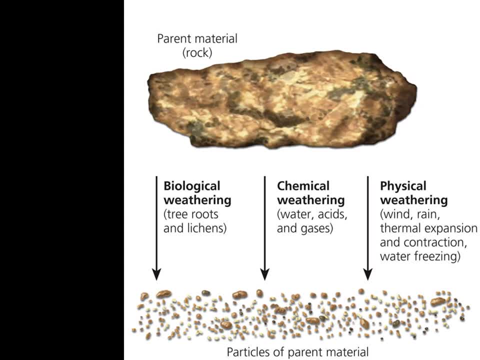 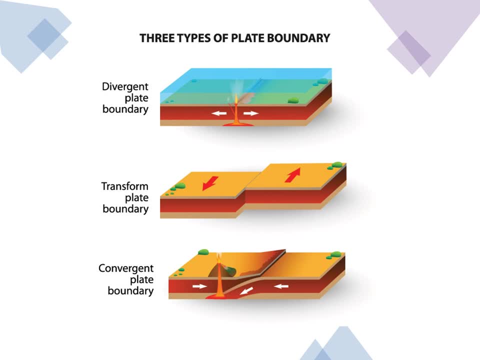 even smaller pieces by plant roots, running water and freezing thawing. The types of boundaries we look at are convergent boundaries, which can result in the creation of mountains, island arcs, earthquakes and volcanoes. Divergent boundaries can result in sea floor spreading rift, valleys, volcanoes. 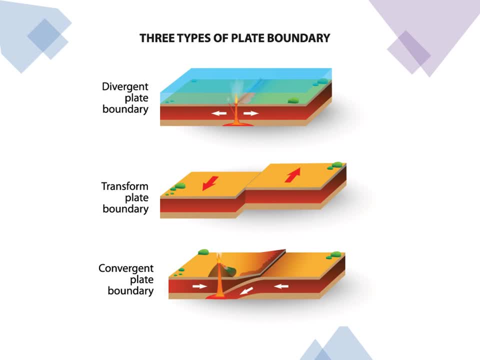 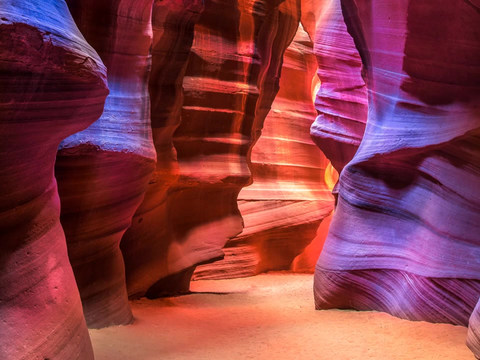 and earthquakes And then transform boundaries which can result in earthquakes. So, convergent run into each other, divergent move apart and transform slight past one another. Another big factor in the geography of Earth is erosion. This is where material has moved from one part of the Earth's surface to another. 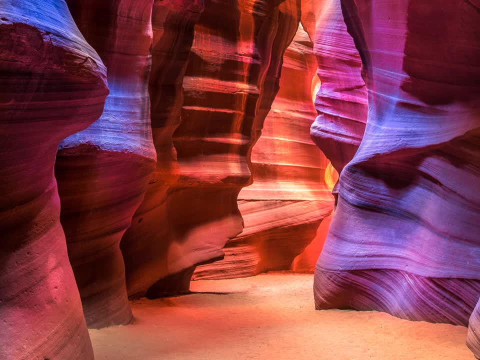 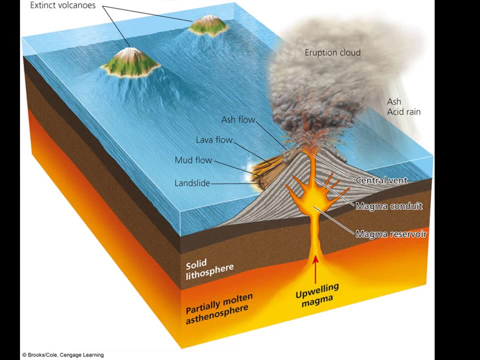 Like when the wind and moving water moving through this canyon carved out this beautiful scene. Let's go back to volcanoes. Those are areas where magma from the Earth's mantle has reached the Earth's surface. Volcanoes have played a major role in the Earth's climate. 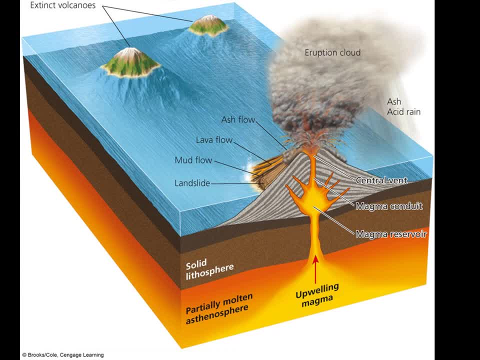 As the smoke and ash they add to the atmosphere can actually help moderate Earth's climate. Some of the ash is so fine that it stays suspended in the air for years, helping to reflect sunlight and keep the Earth cool. Periods of above-average volcanism are linked with cooling global temperatures. 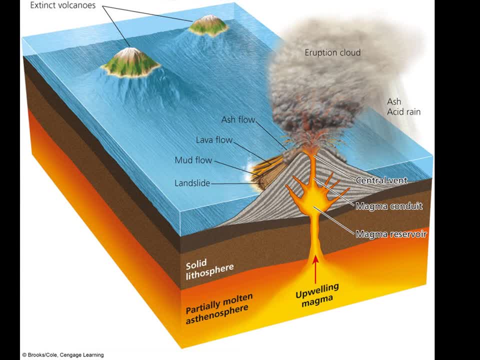 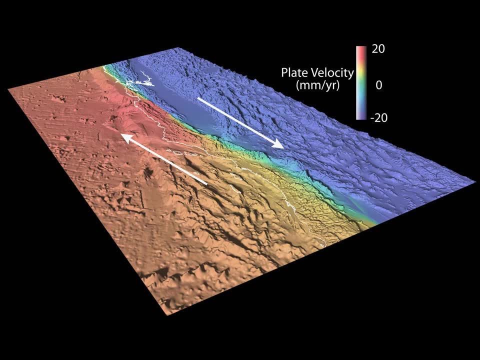 In the period around 65 million years ago when the dinosaurs went extinct was a period of above-average volcano activity. Earthquakes occur when tectonic plates slide past each other but get caught against each other, building up stress that gets released in one large burst. 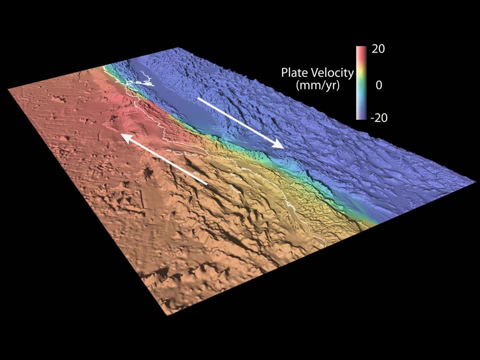 This image of the San Andreas Fault in the western US shows the relative movement of each plate And you can see from the color scale that the maximum movement we're talking about is about 20 millimeters per year, or 2 centimeters per year. 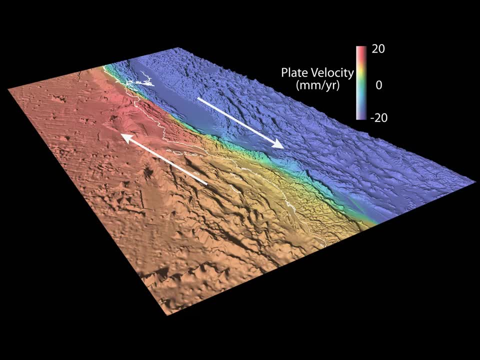 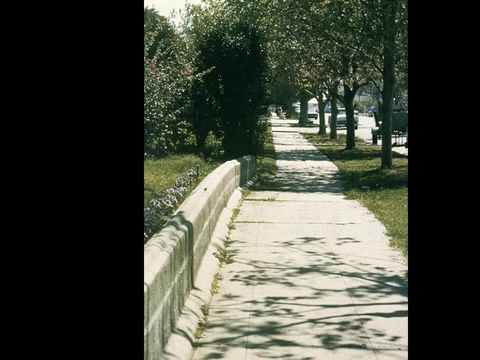 It doesn't seem like much, but it adds up over time. Earthquakes occur when stress overcomes a locked fault. Here's a picture of a sidewalk that straddles the San Andreas Fault as it runs through a neighborhood. When the sidewalk was built, it was straight. 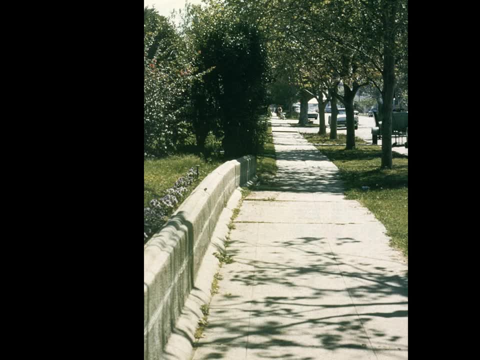 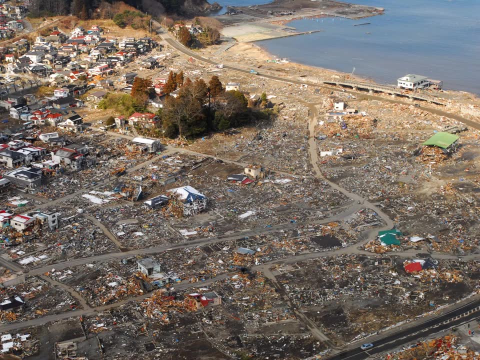 Now, many years later, it's shifted as each plate moves 20 millimeters apart each year. Tsunamis are ocean waves generated from earthquakes that occur on the ocean floor when part of the Earth's crust moves up or down. The movement of Earth's crust may be measured in a few inches, for the actual event. 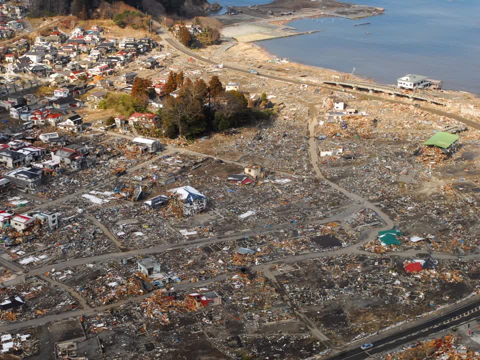 The movement of the Earth's crust may be measured in a few inches for the actual event. The movement of the Earth's crust may be measured in a few inches for the actual event. But as that moving inch of water gets into shallower and shallower water, the height 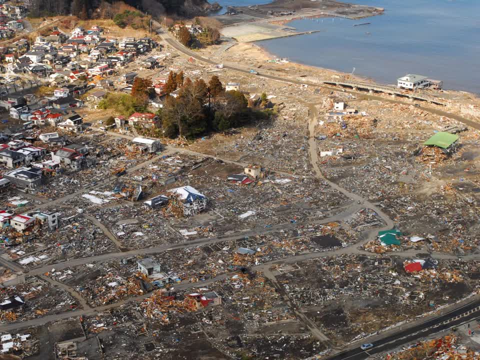 of the wave goes from inches to the height of buildings as it crashes ashore. This picture of the aftereffect of a tsunami shows the destructive power of a wall of water. I'd look very hard for good pictures to make these screen tests, but I couldn't find. 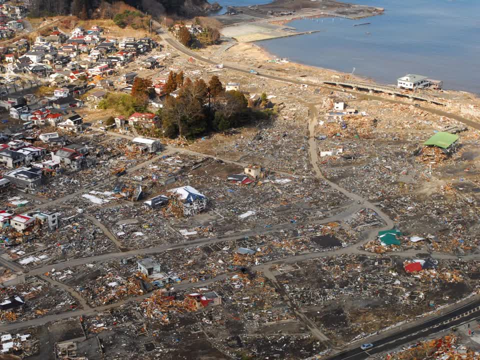 any actual pictures of a tsunami in progress. I attribute it to the thought that most people facing an oncoming tsunami are more concerned for their lives than taking a picture, picking a filter to make it look best and then uploading it to the internet. 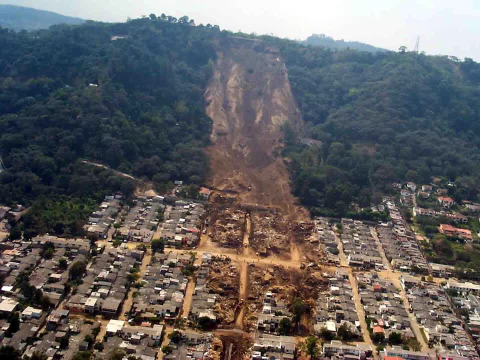 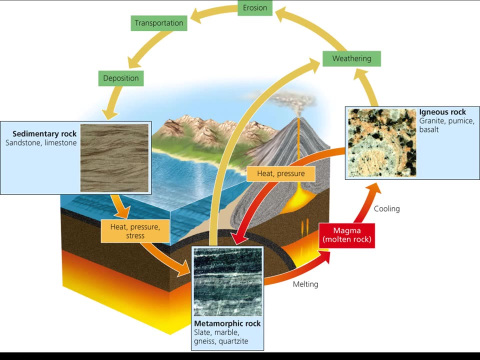 Another geological process is the landslide, or mass wasting. This occurs when huge parts of a hill or mountain come loose in one gigantic flood of soil, rock and mud. Now a bit more about Earth's geology. The last parts of the chapter are concerned with non-renewable minerals. 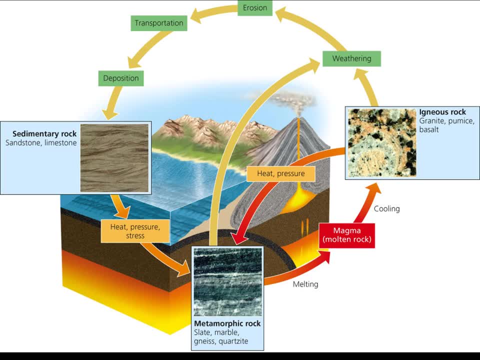 So what exactly is a mineral? Minerals are elements or inorganic compounds that occur in the Earth's crust as they solidify with a crystalline structure. Some minerals are a substance we want directly, like gold, sodium chloride or sulfur, But many minerals are combined with other minerals to form rocks. 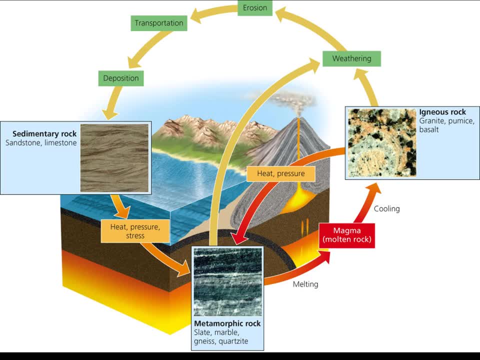 There are three kinds of rocks. Sedimentary rock is made up of fine particles of rock that have been weathered, eroded and deposited by wind or water. As time goes by, the newer layers on top squeeze on the lower layers, compressing them into. 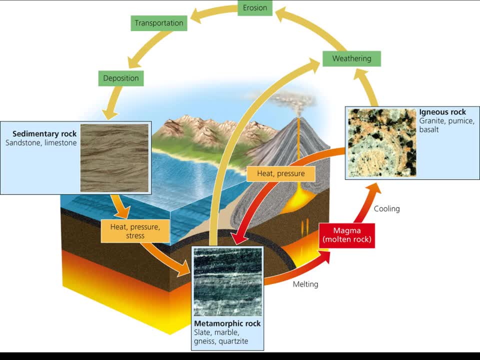 solid rock. Igneous rock is formed when magma cools and solidifies. Metamorphic rock forms when igneous or sedimentary rocks form. This is the most common form of rock. Sedimentary rocks are reheated or subjected to high pressures, causing them to change. 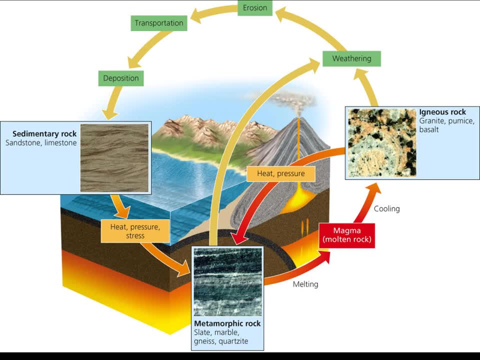 their composition. All of these changes take place over periods of millions of years in the rock cycle, where new rocks are continually being generated as old ones are sort of broken down and recycled. The Earth's crust contains all of the minerals that we use for things in our lives. 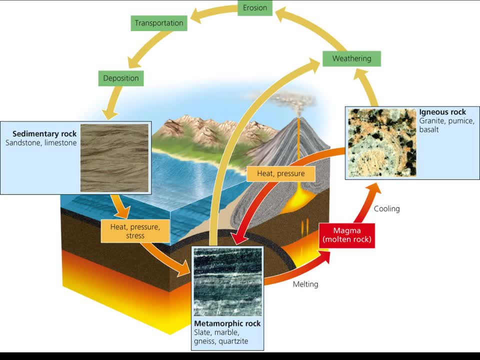 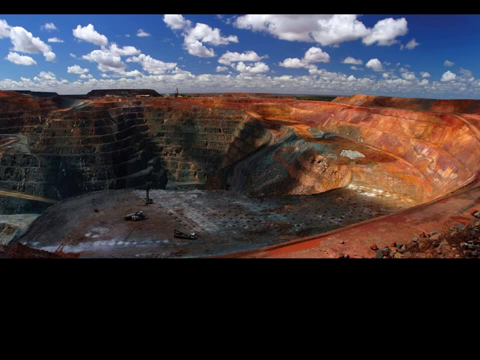 But because it takes millions of years to create new rock material, all of those minerals are going to be non-renewable. Moving on to those minerals, A mineral resource is a concentration of material that can be extracted and processed into useful materials at a reasonable cost. 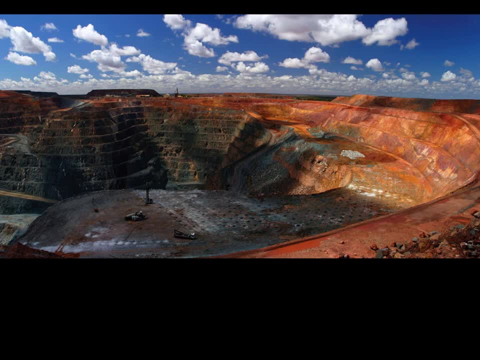 There are minerals that are buried so deep underground or so far under the ocean that the costs of extracting them make them practically unusable. Mineral resources come in three types: Fossil fuels like coal. Metallic minerals like gold, from this mine in the picture. 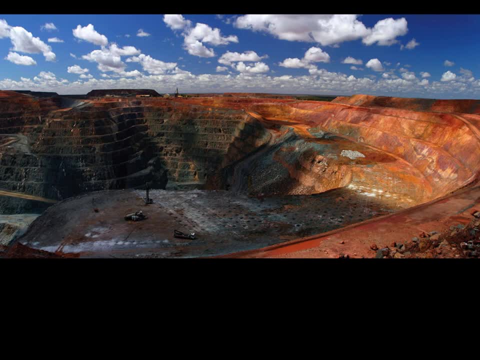 Copper and aluminum, And then non-metallic minerals like sand and gravel. As I said a minute ago, All of these minerals are non-renewable. So what is a mineral resource? A mineral resource is a non-renewable because the process that formed them took so long that 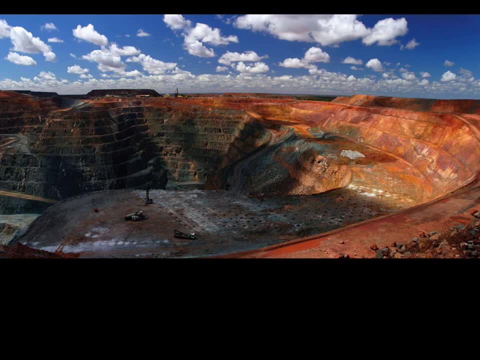 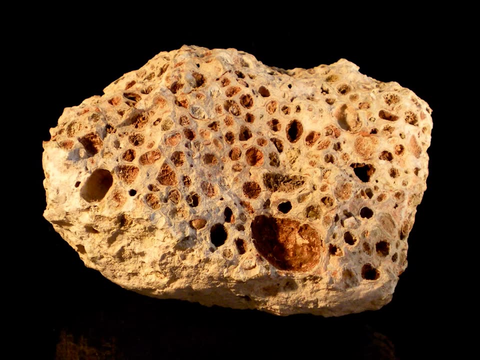 in human time, we've got all that we're going to ever get. Next up is ore. Ore is any rock that contains a useful mineral and a high enough concentration to make it profitable to dig. This is bauxite ore, and it's the type of rock that contains aluminum in high concentration. 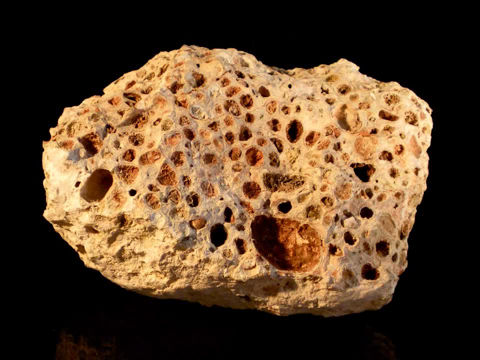 Every soft drink you've ever seen contains aluminum That originally came from a rock that looked like this. High grade ore contains a large amount of this. It contains a large amount of the desired mineral, So low grade ores contain a smaller amount. High grade ore resources are usually extracted first because it's much more cost effective. 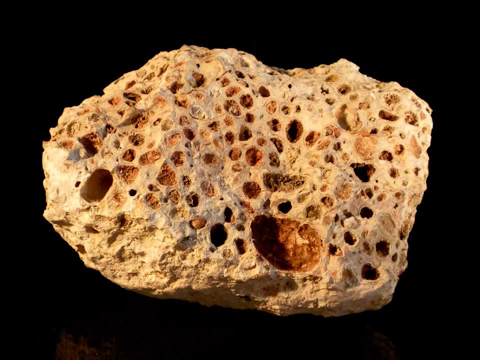 By this point in human history, geologists from every country have determined estimates of how much each mineral resource exists. Those estimates are of the reserves, and they're called that because they are resources that have yet to be extracted. They're called that because they are resources that have yet to be extracted, and they're 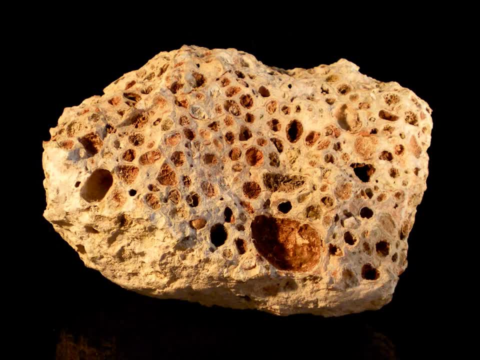 called that because they are resources that have yet to be extracted. and they're called that because they are resources that have yet to be extracted. So, this is bauxite ore, and they're called that because they are resources that have yet to be extracted. and they're called that because they are resources that have yet to be extracted. 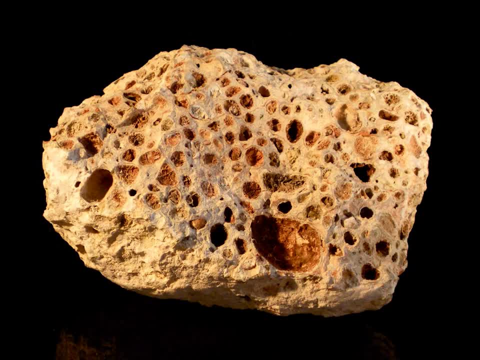 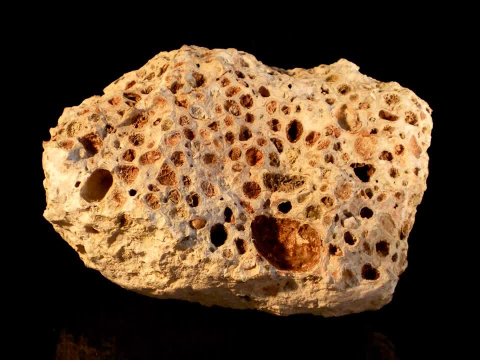 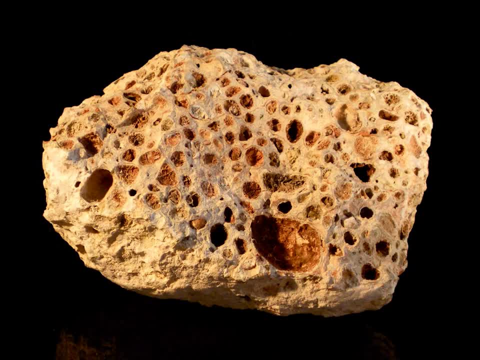 So these estimates have changed over time as newer techniques have led to identifying new reserves and a newer technology has allowed previously inaccessible reserves to be extracted. But no matter how you estimate it or what tools and techniques there are to use, there is a fixed quantity of each mineral resource on Earth. 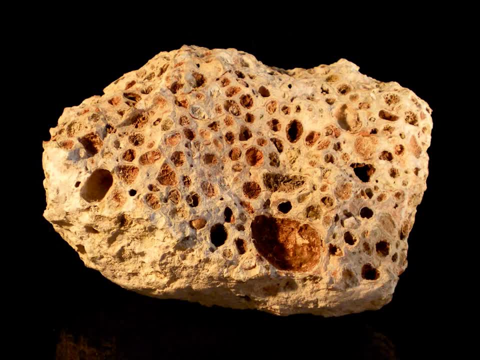 We're limited to what we have here. There are many examples of mineral resources in your notes. As I mentioned the first one, aluminum has been important for soft drink cans, and now I'll tell you that aluminum is also an important building process for burning coffee tea. 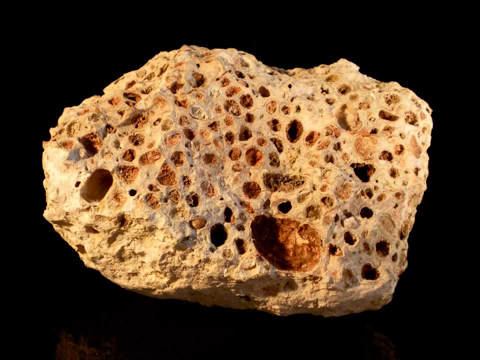 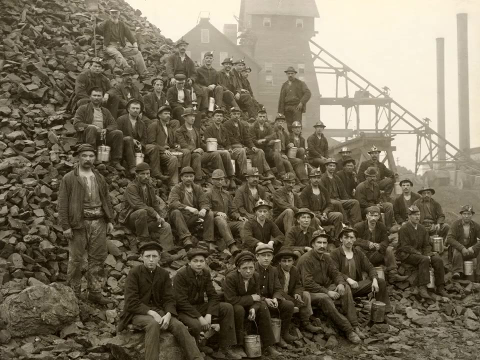 important building material. For a while it was used as the electrical conductor in wiring, but that was a disaster. So now wires are made of copper, But you need to read through the book and find what each of the other mineral resources is used for. There are many advantages and 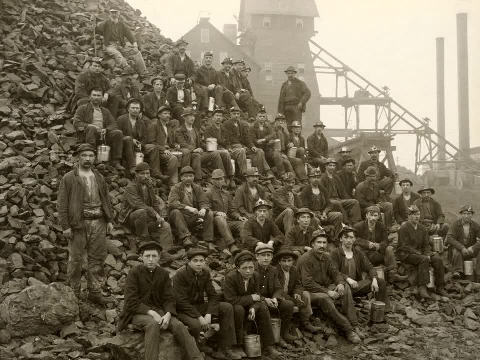 disadvantages to mineral use. First up, mineral resources are incredibly valuable for the country they're founded. Mineral resources bring money into a country by furnishing raw materials for many industrial products that will be sold to other countries, And they also help create jobs, as the minerals are extracted by these miners, processed and used in industry. The disadvantages: 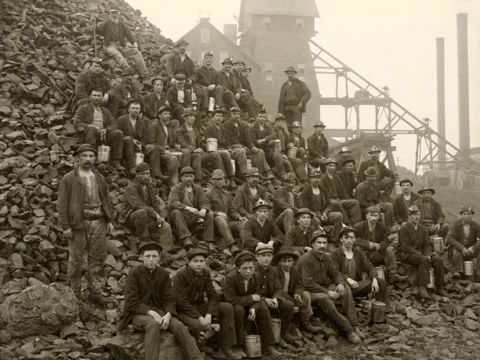 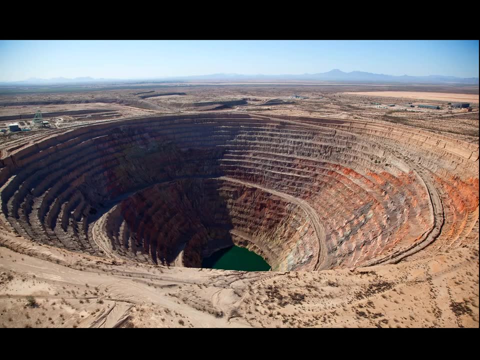 are numerous because the process of mining, processing and refining minerals is very hard on the environment. There are two big ways to remove mineral deposits from the earth so that we can be used. First up is surface mining, which is sort of top-down approach. The rock material: 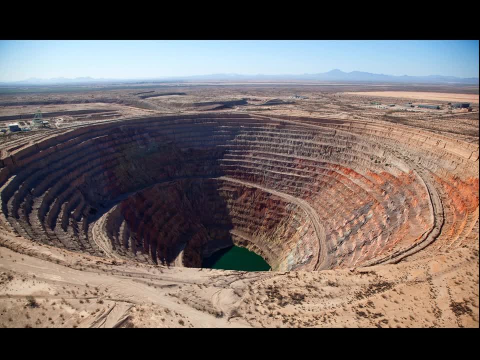 that covers the earth is used to mine minerals And it's used for mining the earth And it's desired deposit of minerals is called overburden and it is removed and dumped off site and is called the spoils when it is removed. Tailings are another form of spoils where rock that previously 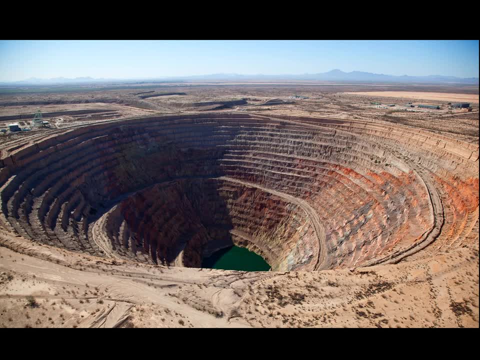 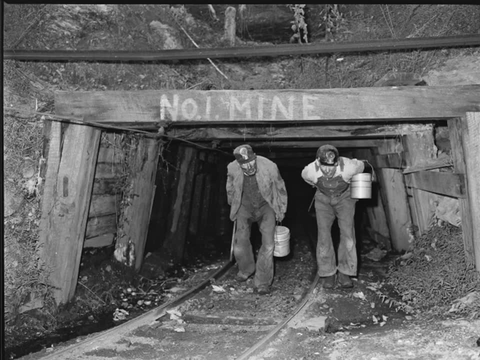 contained minerals is left behind on the surface after removing the minerals from it. Subsurface mining is a bottom-up approach where shafts are dug underground to extract mineral resources. The path of the mine follows the deposits as they run underground and the overlaying material is left in place. There are many harmful effects of mining and extracting. 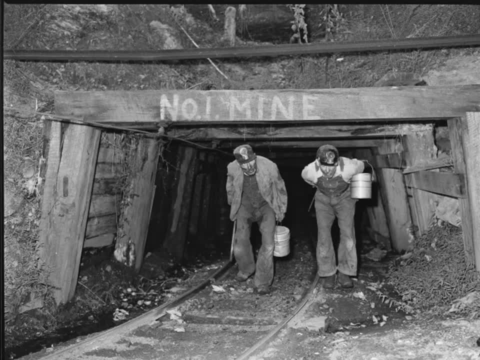 minerals. First, surface mining completely removes whatever natural ecosystem was in place before the mine was constructed. Second, the mining spoils topsoil, so new plants have a hard time getting established in areas where the tailings are dumped. Third, chemicals that the tailings 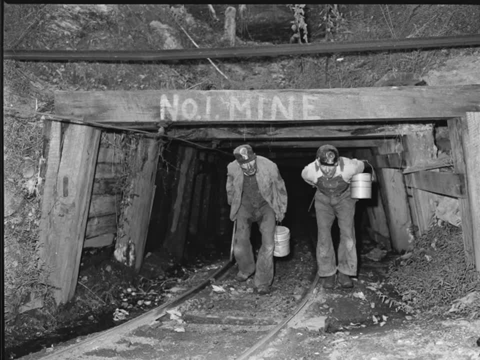 contain are easily washed out by rain and find their way into rivers, streams and lakes. Those chemicals may not have been big problems when they were under ground, but when released in huge quantities above ground, they can cause environmental havoc Last up. the process of extracting the mineral from the ore it's contained in is called smelting. 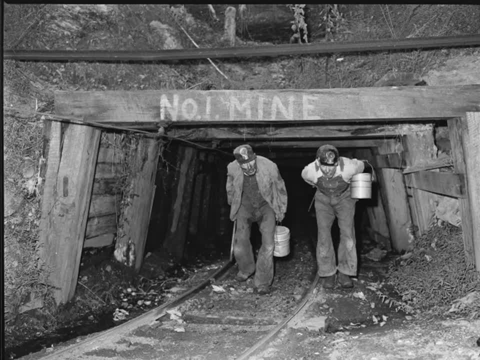 Smelting occurs when ore is heated and chemicals are added to release the minerals. This can result in massive amounts of air and water pollution, as some of those chemicals are released into the environment. As things like coal reserves get smaller, it becomes necessary to mine coal through. 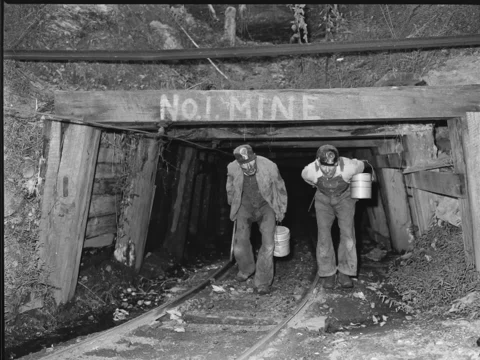 subsurface mining. As coal reserves get smaller, it becomes necessary to mine coal through subsurface mining. As coal reserves get smaller, it becomes necessary to mine coal through subsurface mining, Which is very expensive. Plus, as more reserves are depleted, we must 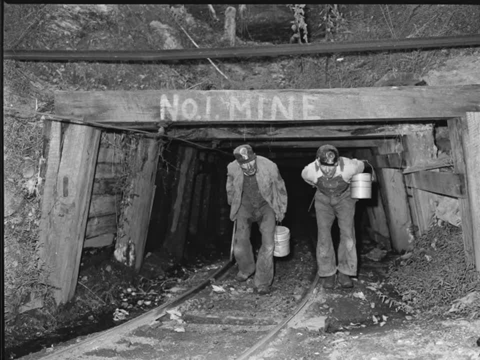 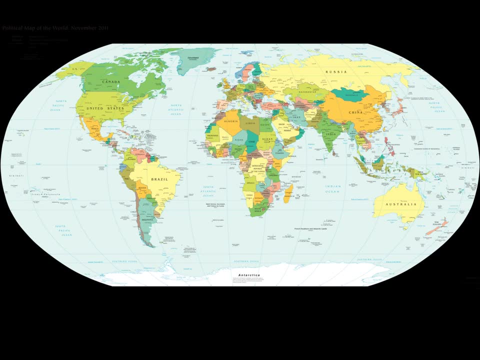 also access lower grade ores, which leads to more pollution when using them. Now, if all mineral resources are, by definition, non-renewable, how long will the supplies we have last? I like to think that the answer is long enough, because when we've used up enough of it that prices start to rise, we as a society will shift, and 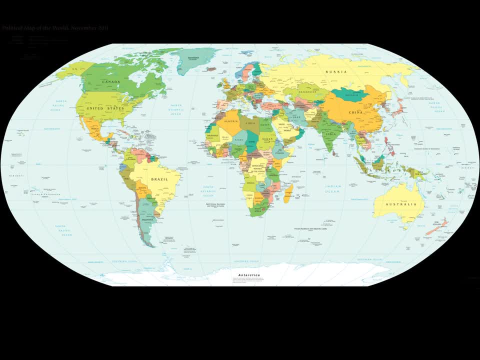 find alternatives or start seriously recycling what we have in order to make it last. There won't be a day where there suddenly is no more iron to make steel, but there will be a day when we have many alternatives to steel and the steel from cars and old buildings will be recycled. 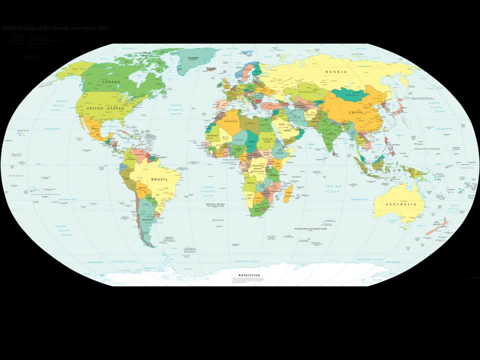 much, much more than it is today. Now I have a world map up here. because of the idea of mineral distribution, Different areas of the world have different amounts of these resources, so minerals are distributed unevenly over the surface of the earth. Some countries have a more complete set of resources. 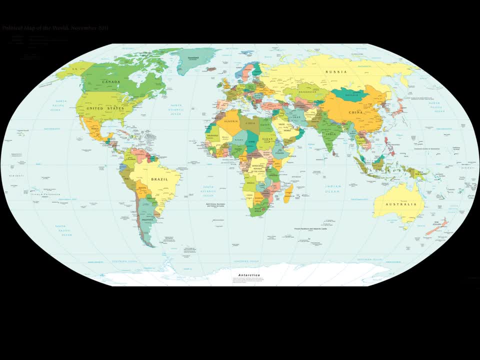 others are heavily dependent on trading with mineral-rich countries. Economic depletion occurs when a mineral costs more to find, extract, transport and process any remaining resources than it's actually worth. After economic depletion, there are five alternatives to use using new minerals. First, reuse and recycle existing supplies. then waste less, then use less. 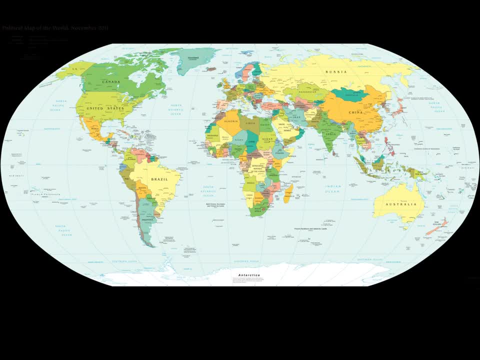 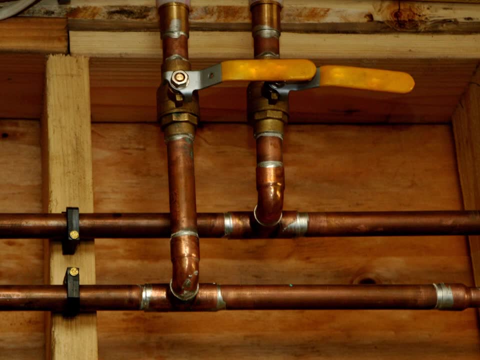 substitute it or you just do without it. Substitutes are a great way to reduce current levels of consumption of some mineral resources. This copper plumbing used to be very common in all types of buildings, but as copper resources have been overused in recent 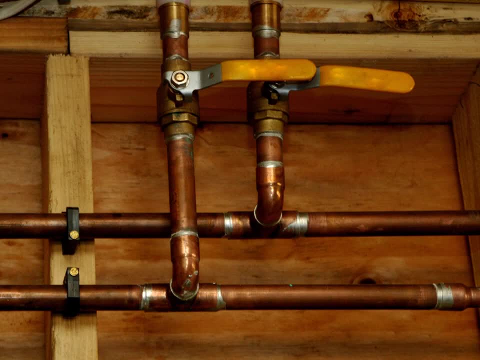 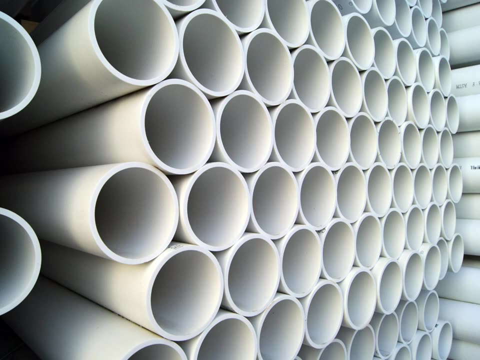 decades, and the price of copper has increased dramatically. it's been replaced by PVC or plastic tubing. Now the oil used to make this plastic is also non-renewable, but let's save that for a later chapter. The US government stopped minting all copper pennies. 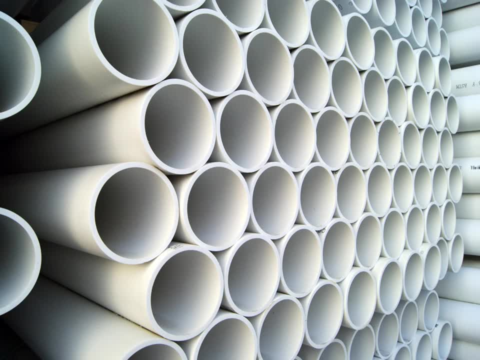 in 1982, and since then they're made of mostly zinc with a light copper coating. It's funny that if you have a penny minted before 1982, it's actually worth about 2.5 cents for the copper it contains. It's a pretty safe way to double your money, as people actually go to the. bank and purchase large amounts of pennies, sort through them and keep all of the copper ones and return all the later ones and repeat the process. They're keeping all of the copper ones and one day, when the price of copper skyrockets, they'll trade all of those pennies to a copper. 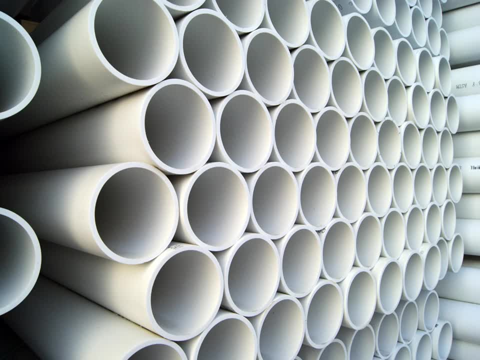 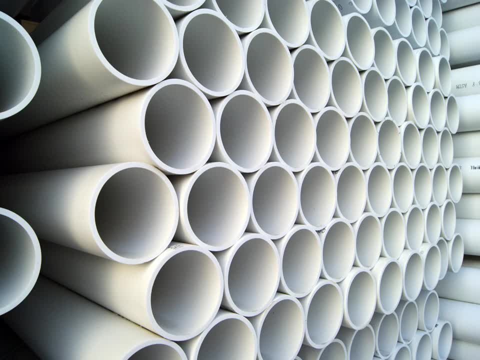 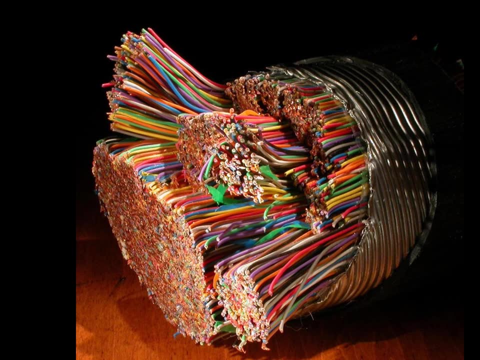 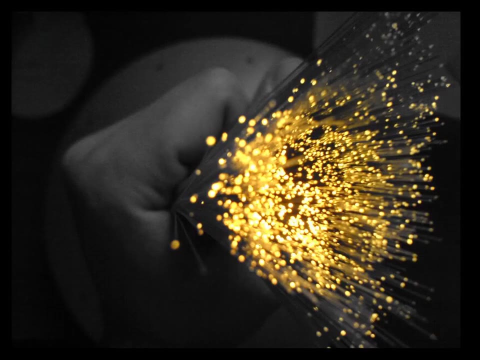 Let's get started. Let's get started. It's kind of an interesting idea to make a little money. Replacements for copper wiring, like this ancient telephone trunk line, have also been developed, such as modern fiber optic cables, which have been developed and used. Now that's made out of plastic too, which is also non-renewable. 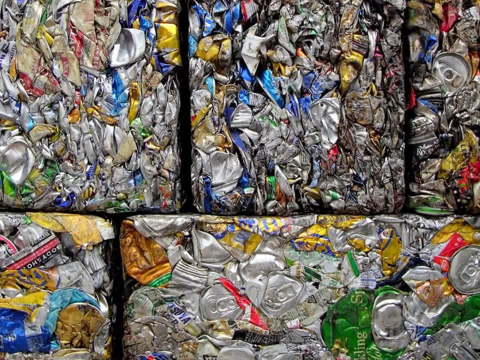 So in the recycling and reusing department we can greatly extend the time we have left with most mineral resources Simply by recycling them or reusing them before they have to be recycled. The financial and environmental cost of recycling something like aluminum cans is tiny when compared. 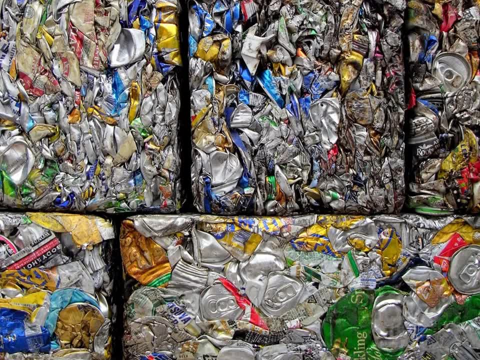 to the cost of extracting raw materials from the earth and processing them into new aluminum, And it's a process that can continue indefinitely. At the going rate for aluminum in 2023,, a single aluminum can is worth between 5 and 10 cents for the metal it contains. 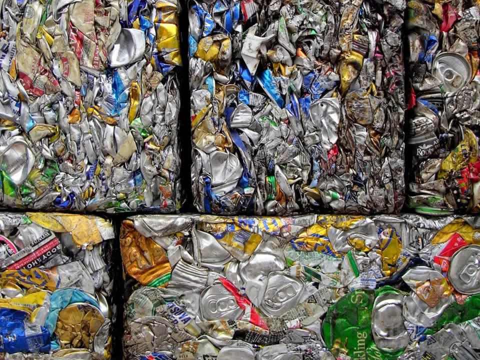 So not recycling a whole 12-pack is like throwing away between 50 cents and a dollar. It's not going to send children to college, but I have a huge trash can filled with crushed cans and it's nice to take it to a recycler once a year. and you know get you know.